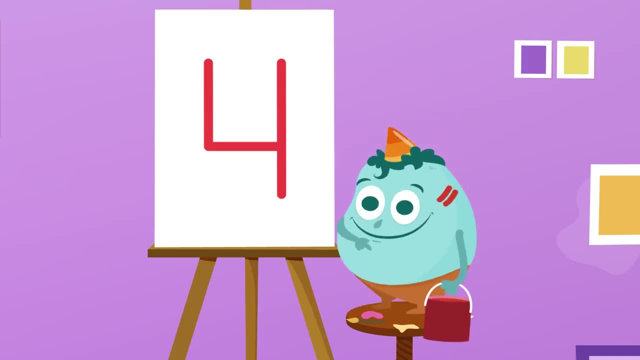 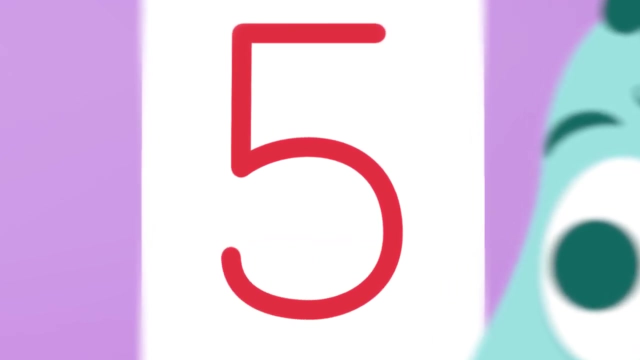 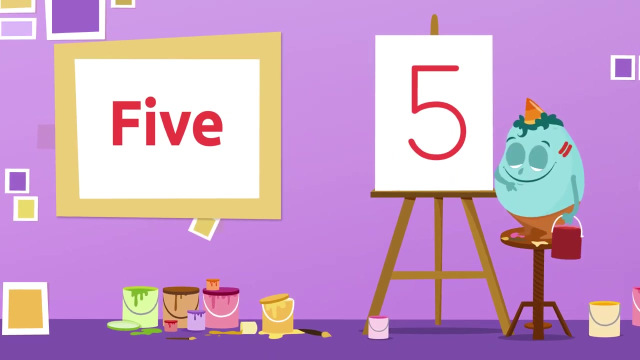 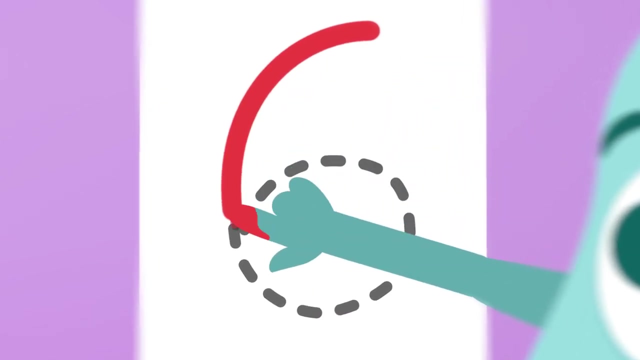 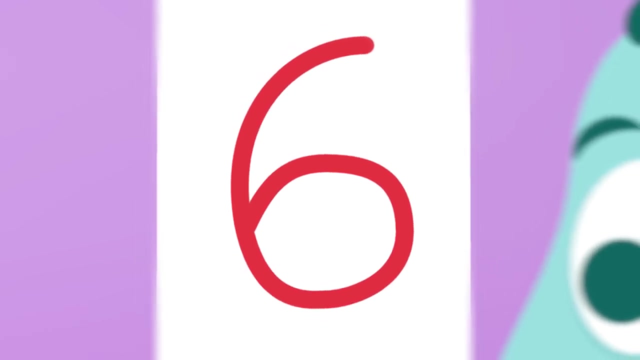 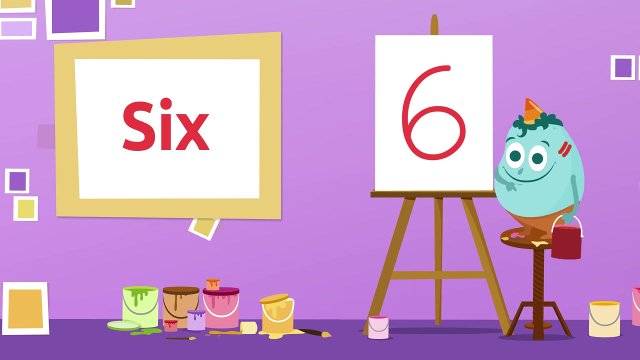 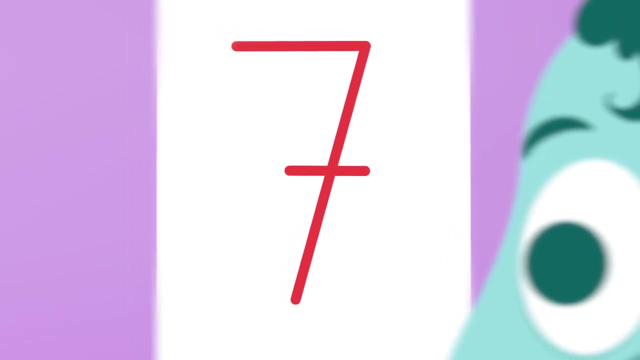 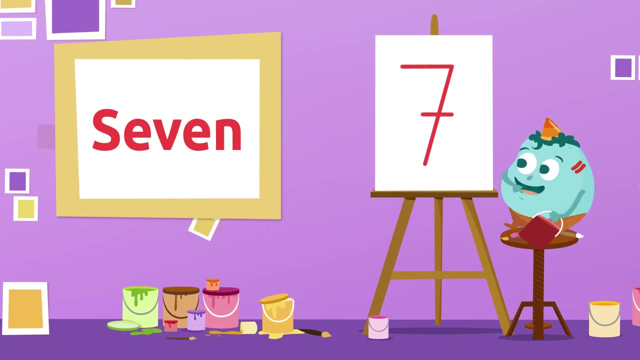 Way to go. Number four: Four. Let's try the next one. Which number is this? That's it. Number five: Five. Let's see if you know which one comes next. Let's see. This number is Yes. This is number six, Six. And the next one, Which could it be? And this one, Which number is it? Good, This is number seven, Seven. 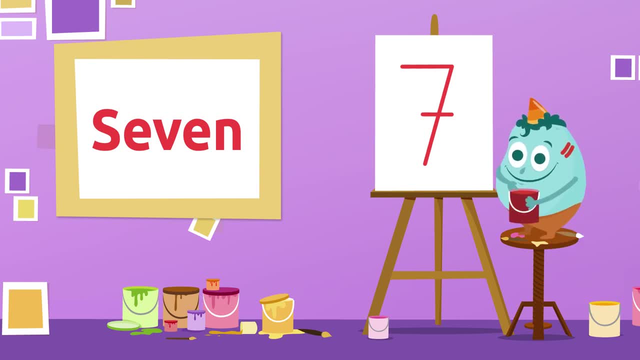 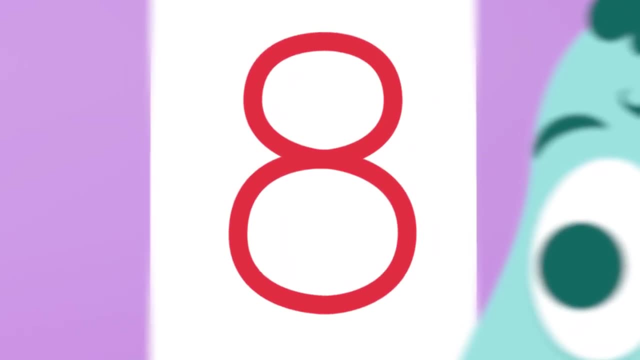 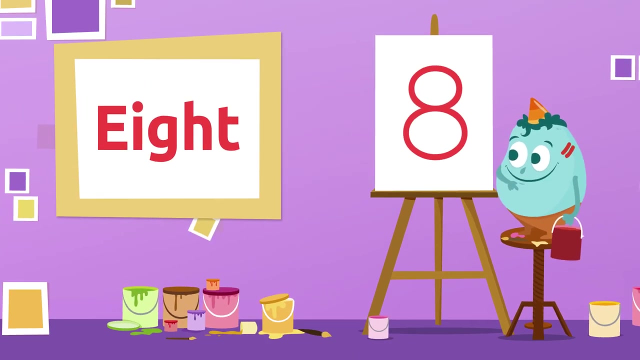 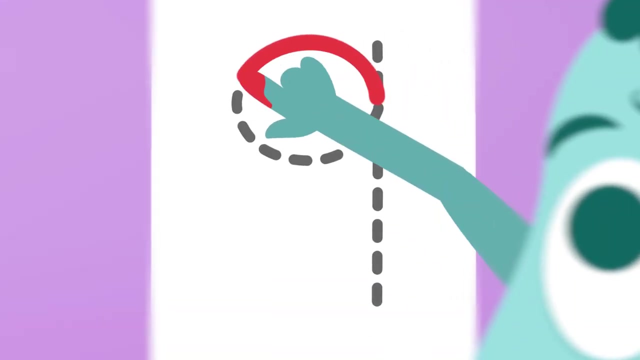 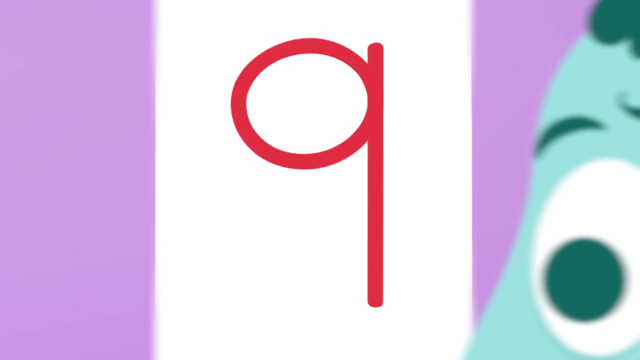 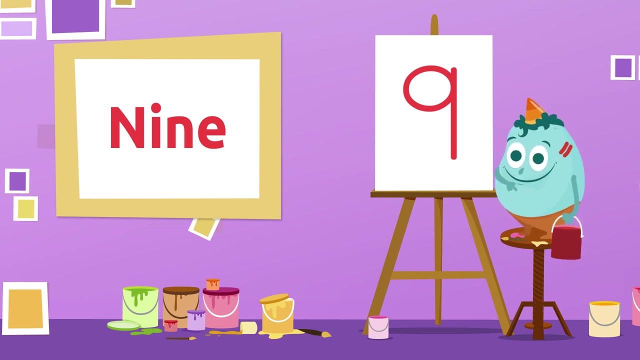 Will you guess the next one? Which number is this? You aced it. This is number eight. Eight, You're doing great. Which number have we got here? Number nine, Nine, So good, This is number nine Nine. 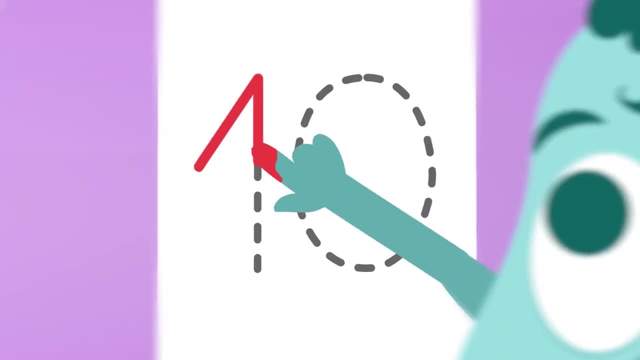 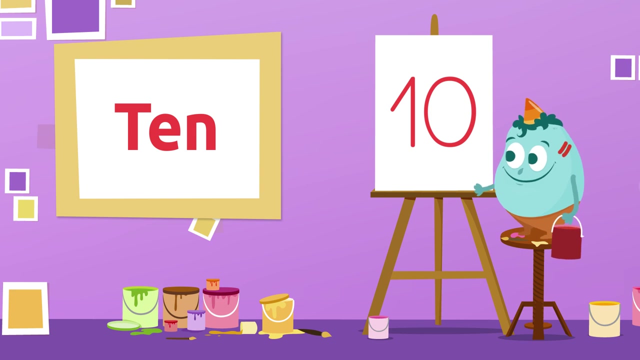 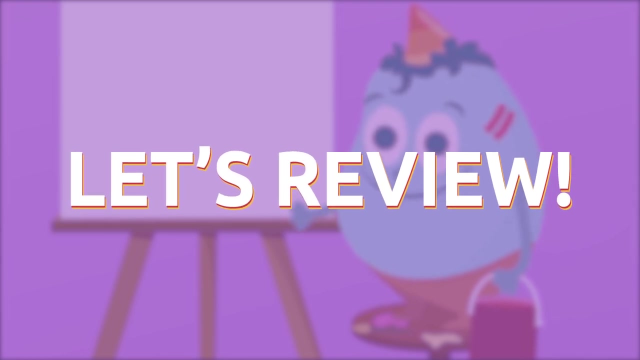 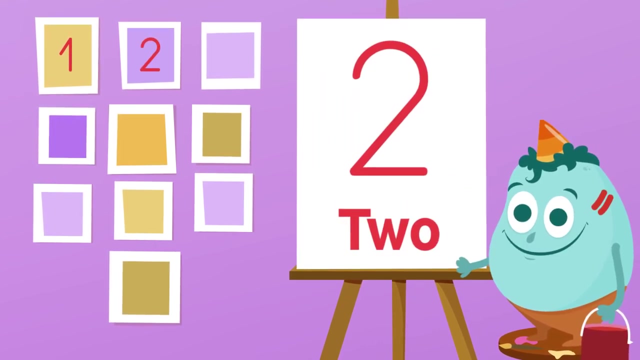 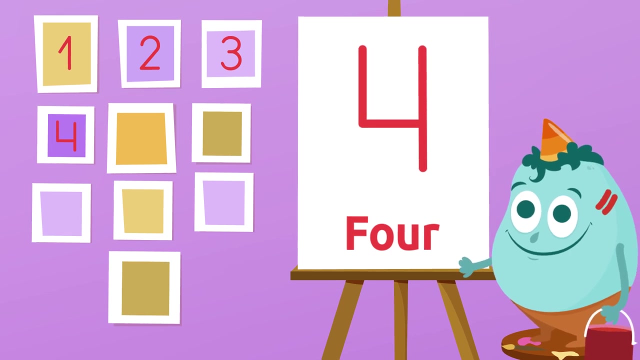 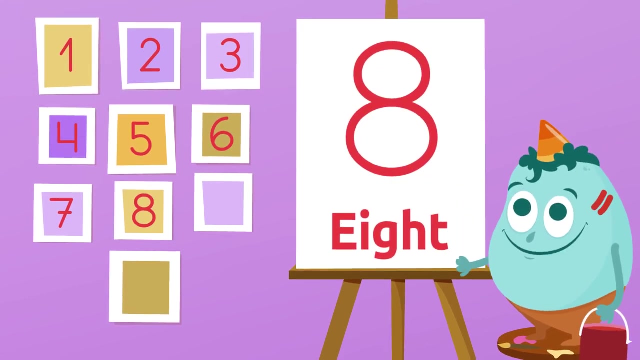 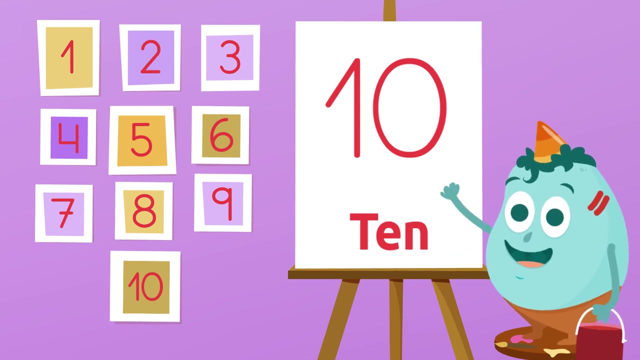 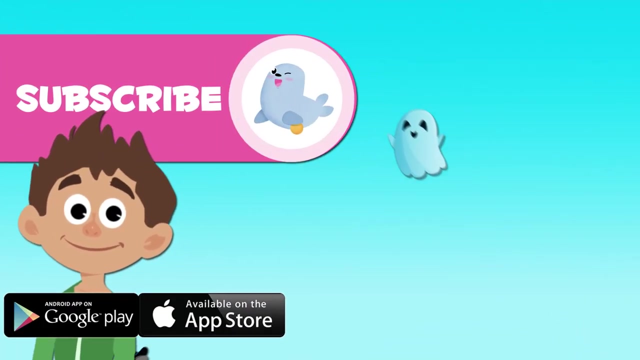 And the next one. Will you know which one is it? What is this number? Well done, This is number ten Ten. you did great. one, two, three, four, five, six, seven, eight, nine, ten. well done, Bravo. do you like this video about numbers? there are. 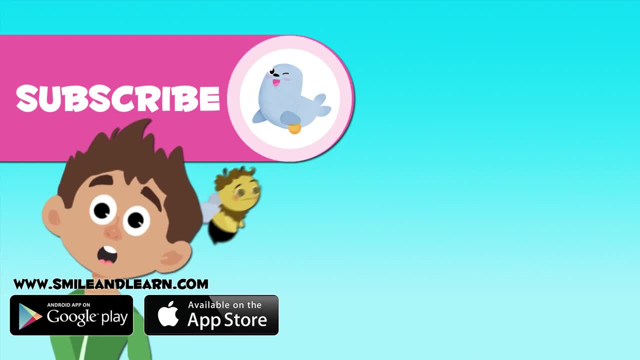 lots more. click on the seal to subscribe to the smile and learn. YouTube channel you.